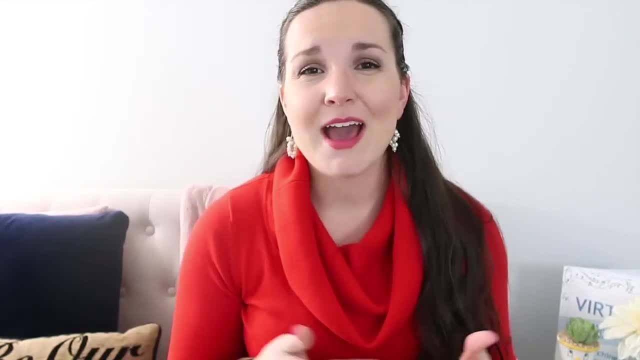 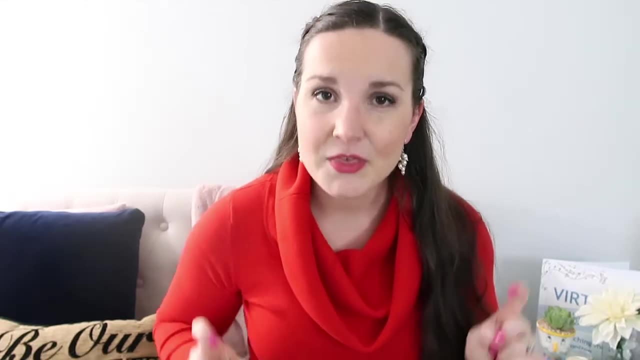 know having to make these decisions that, honestly, they just shouldn't have to do. then having this safe space in the music room where they can play and be a little more little kiddish is great. With that said, we're going over movement activities today, and so some of them you might be like: oh. 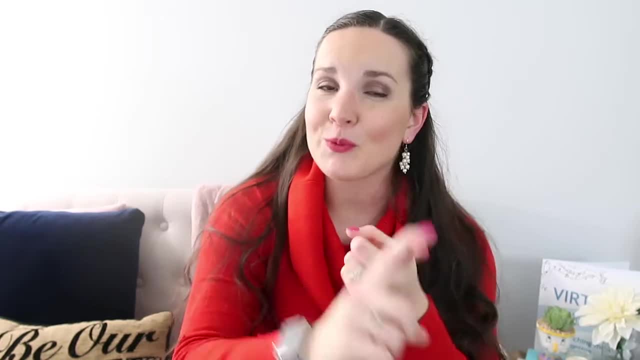 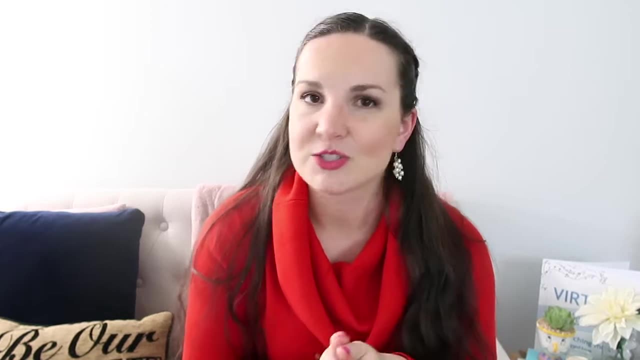 my fifth graders won't like that, but I promise, if you approach it the correct way and if you enjoy it and if you, you know, make it seem like they're gonna enjoy it, they will love it because they are so much fun. If you enjoy this video, please make sure you hit the like and the subscribe button. 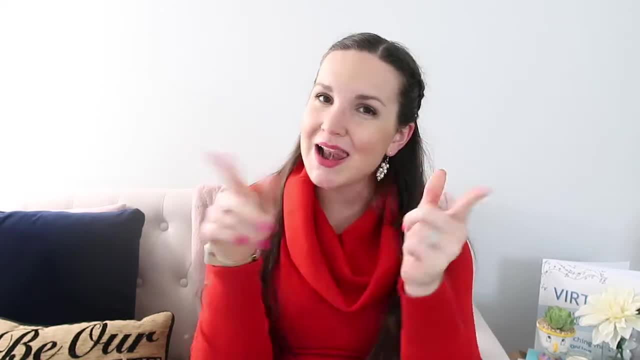 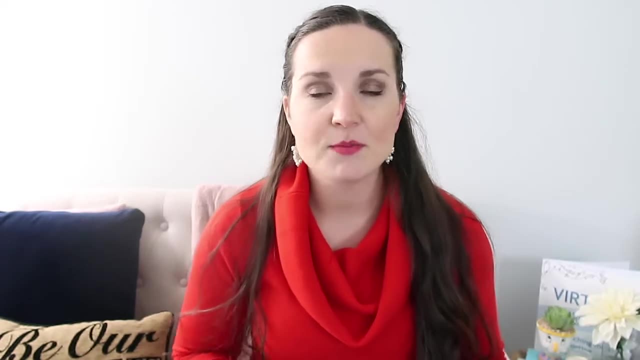 that really helps me out. so, without further ado, let's hop right on in. All right, all of these are like really simple ones that you can do pretty much any time of year, pretty much for any concept, for any, just anything, anything. they're really simple and they're fun. So my first one is called: 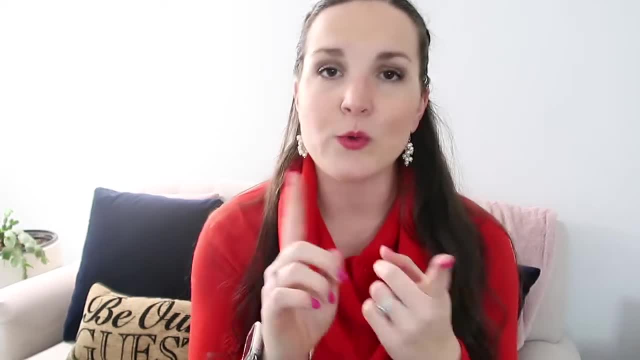 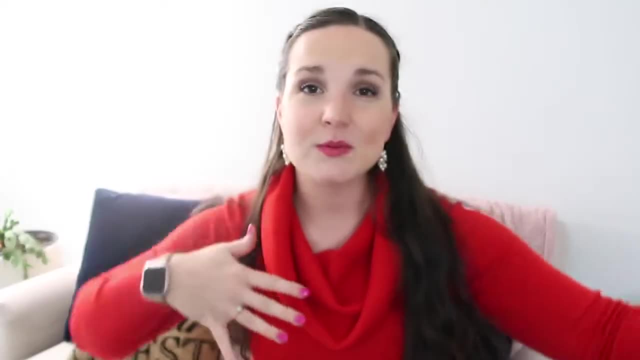 rhythm stomp. This is one of my favorite ways to incorporate reading rhythms and also moving our bodies. So what we do very, very simply is, instead of clapping rhythms or saying rhythms, we put them in our feet. so this requires the kids to stand up and they stomp it. If you want to have 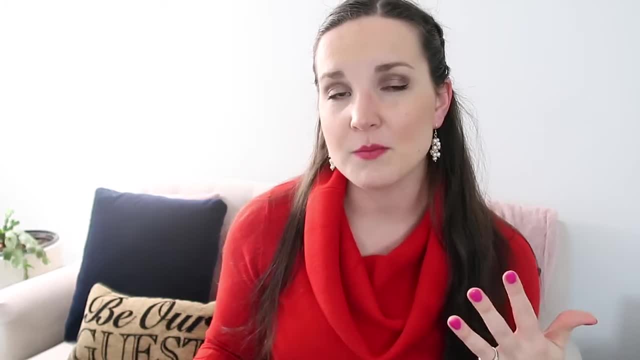 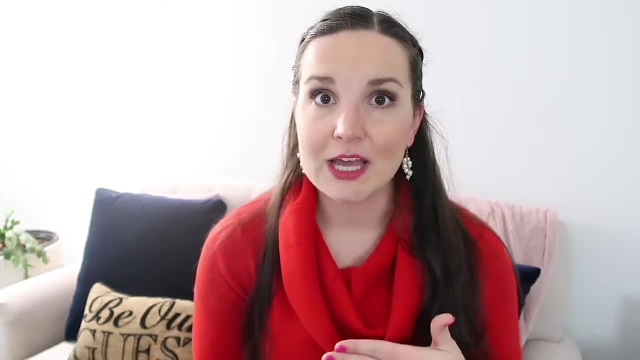 a lot of fun. you can change the different places where they're going to keep the, where they're going to play the rhythm, so they could like snap one, clap one, stomp one, all of those different things. I've also seen quite a few play-alongs that are body percussion play-alongs on YouTube. 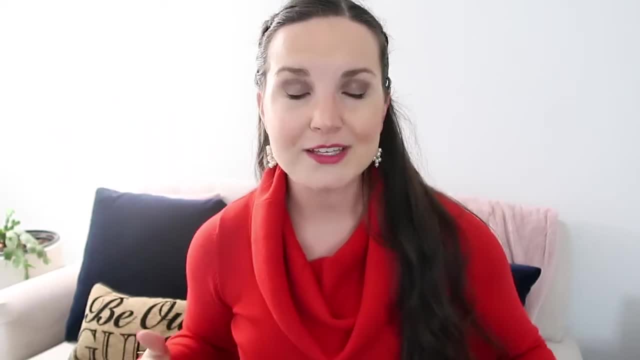 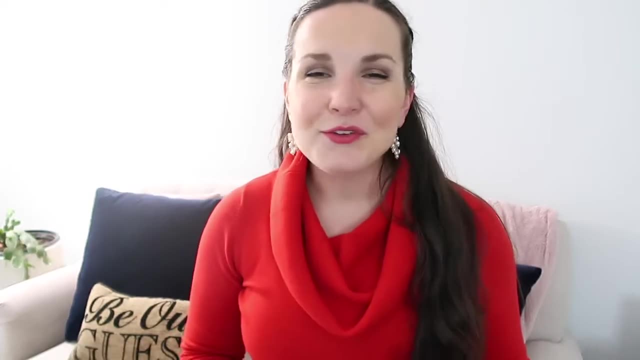 that are a lot of fun and get kids reading rhythms and also moving like their whole body. so you can definitely check those out. just search body percussion play-along and you'll find it. it's pretty simple and there's a lot of really fun ones on there. that might be a little bit more. 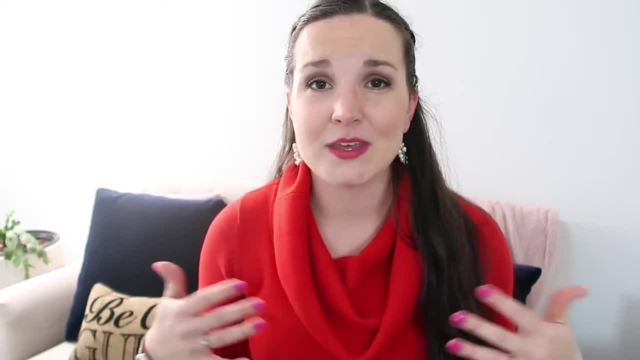 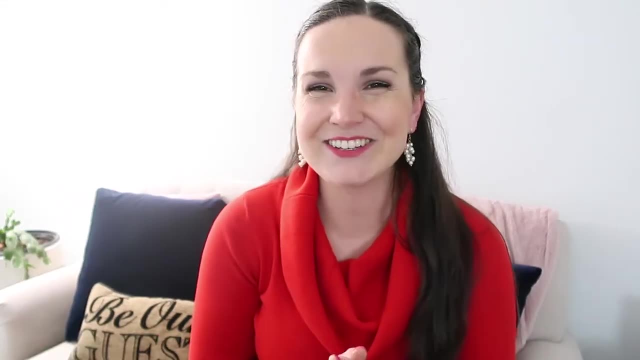 if fifth graders have loved. But you can even do this just with, like you know, old school rhythm cards. remember when we like printed things out? No, Well, you can, and you can still use those, and they work just fine. Number two is one you're probably sick of hearing me talk about, and that 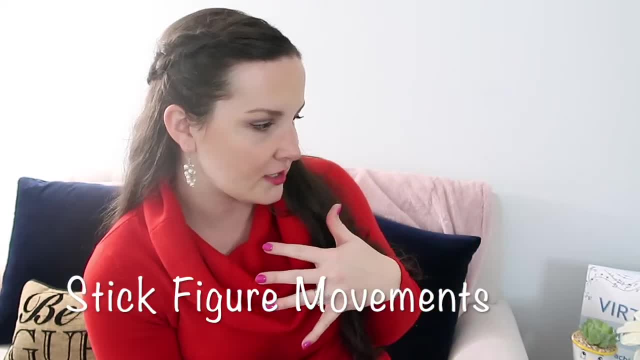 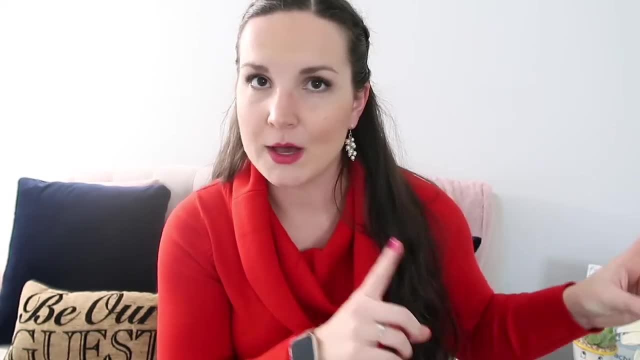 is stick figure movements. Now, I thought I had some stick figures printed out, but apparently I don't. You know, I'm not gonna lie, it was really convenient when I was teaching online from my house for these videos, but now that I'm teaching online from the school, I'm teaching online from 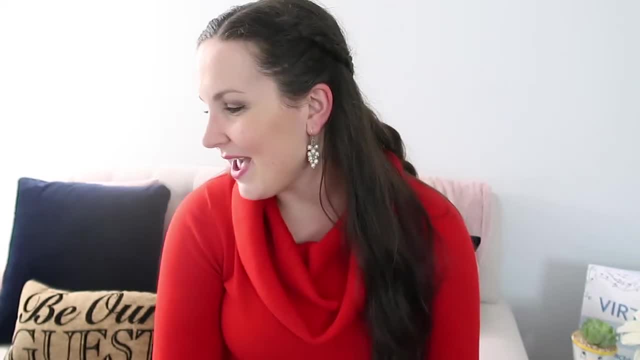 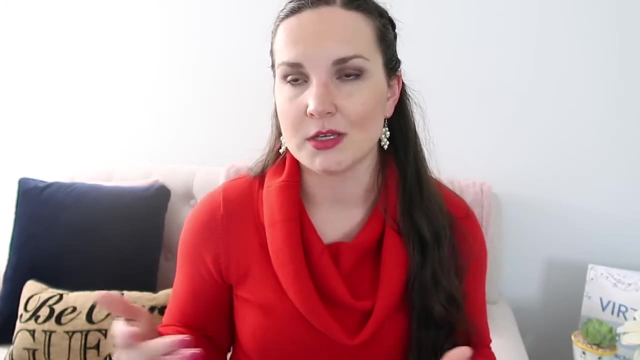 school, my stuff. I keep forgetting to bring things home. So anyway, regardless, stick figure movement is really fun. I love to use it like the first week of school, and usually again in January and anytime I want them to listen to something they might not like, and so basically all you do is you. 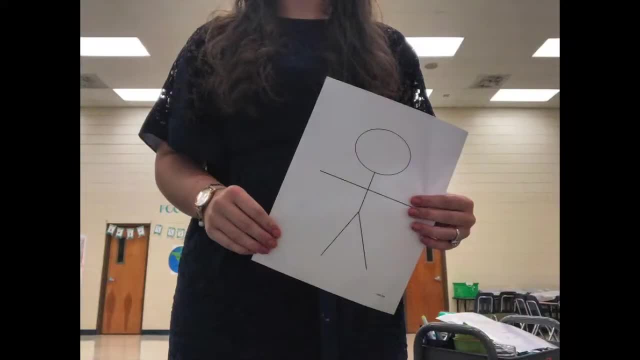 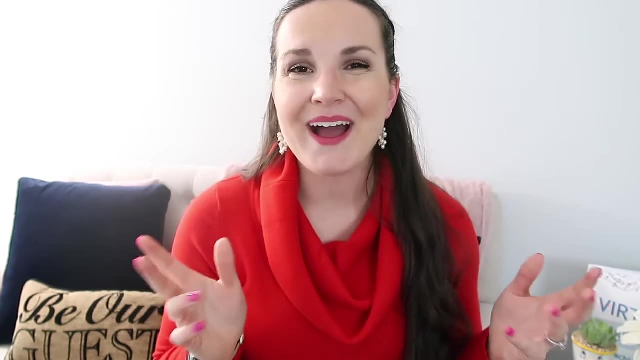 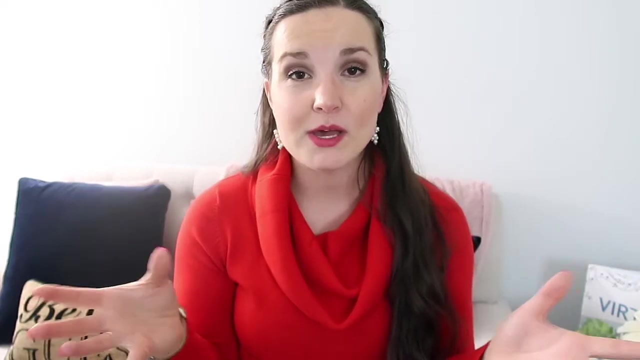 have some papers that have different stick figure shapes on them. I have some in my TPT shop. I will link below. They're super cheap- I think it's like the cheapest thing in my store. So all you do is match the stick figures movement So you can make any different ones. You can do like partner ones. 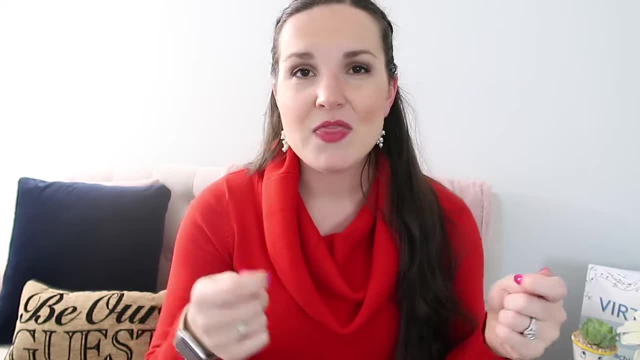 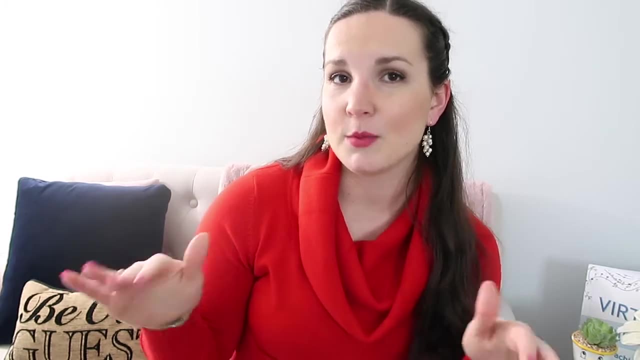 or three people ones, whatever you would like to do, and then I just change them, usually like every four beats, To make it a little more interesting. I love to add like backing tracks, so you know, like hip-hop backing tracks, or you can also add just any kind of music. This is a great chance to add. 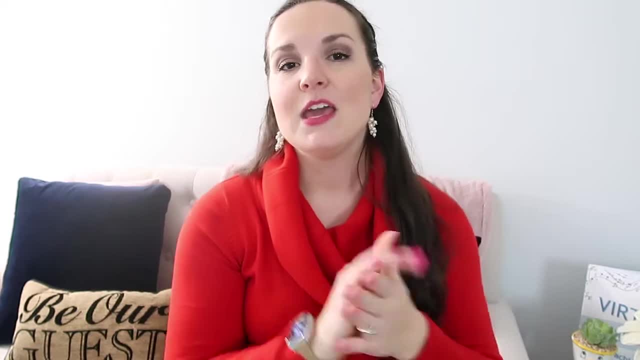 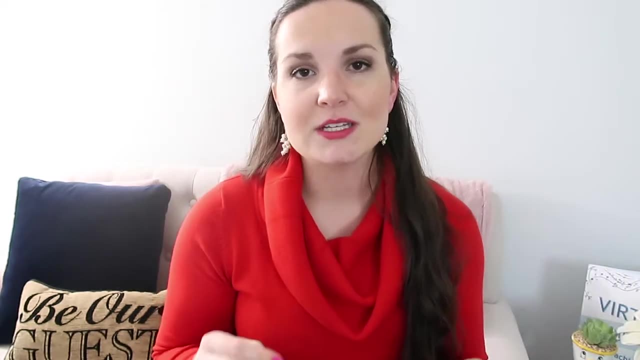 maybe some music you wouldn't normally play, or if you're doing a lesson where maybe you're listening to some music that the kids might not be sure about, It's a really good way to get them to listen to something in like a safe environment, so it's not like 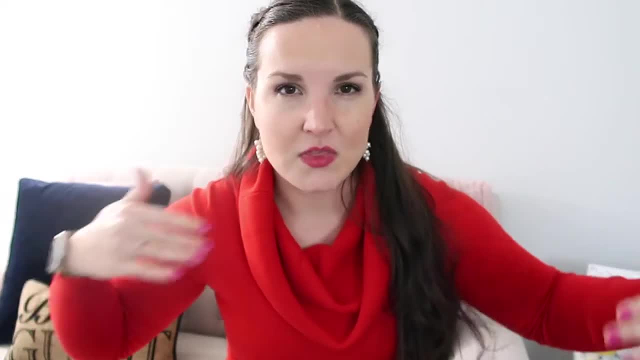 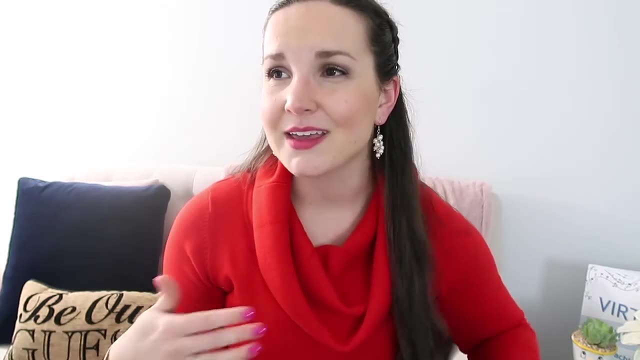 what the heck is that? It's like: oh, I'm, you know, focused on this, and then the music's just kind of there and they don't realize it at first. It's also like: maybe, if you want to incorporate a pop song- I know I like the idea of incorporating pop songs, but I have a really hard time figuring out- like: 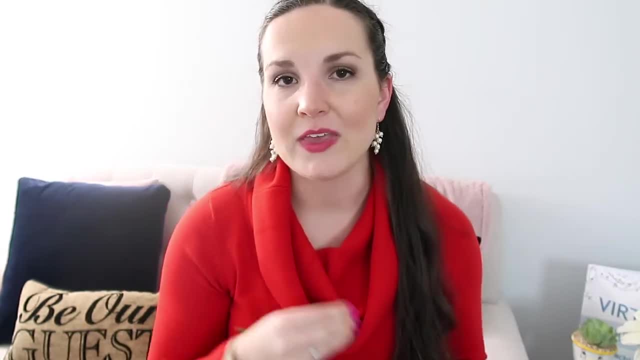 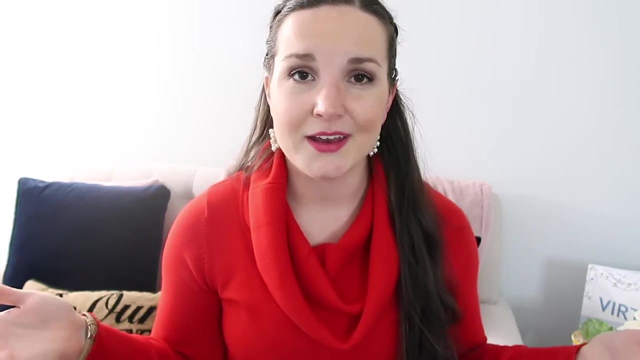 actually how to put them in my curriculum. This is a really good way to do that, like as a nice warm-up at the beginning, or if you want to feature like different songs from different people, you can, and that's fine too. It's extra fun when you um switch up the pattern after a while, so sometimes 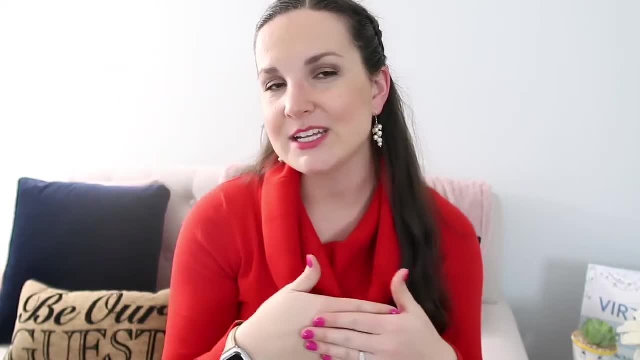 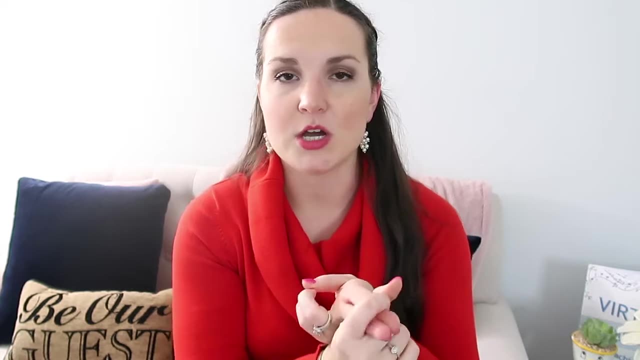 I'll start going backwards or I will also put like a blank one in, so when you get to the blank one, then you can make up whatever you want. Super fun. I will leave a link to both my stick figures and a blog post where I talk about like four or six different ways that you can use the stick figure. 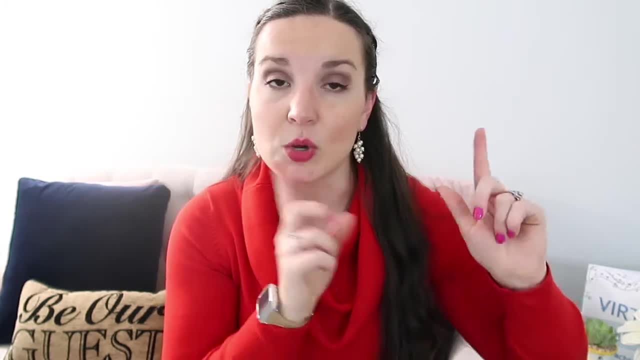 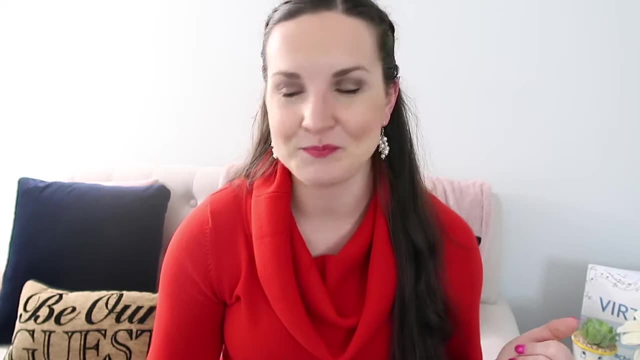 movement cards. so click the link below and check that out, because there's a lot of different things that you can do and they're so simple and so easy and so much fun, All right. the next one is another way you can incorporate some of your pop songs, or just for. 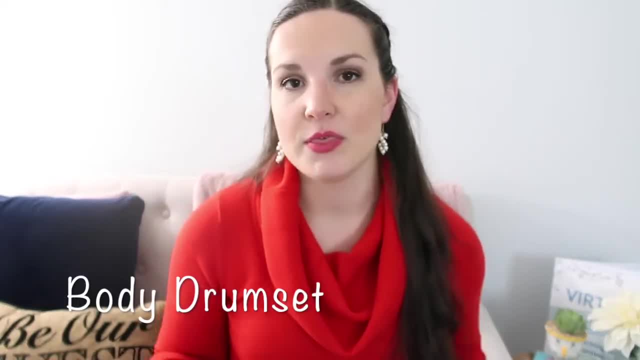 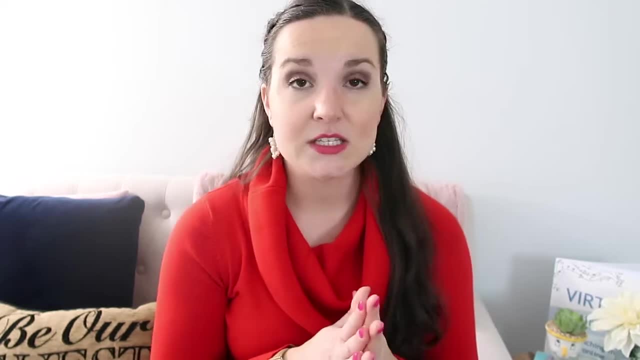 fun and that is body drum set. So this is one that I learned from Little Kids Rock. I will link their website down below. Actually, I will link the particular song we used. So we did the song Counting Stars along with this and it was really easy, which is why I picked it, but it was also 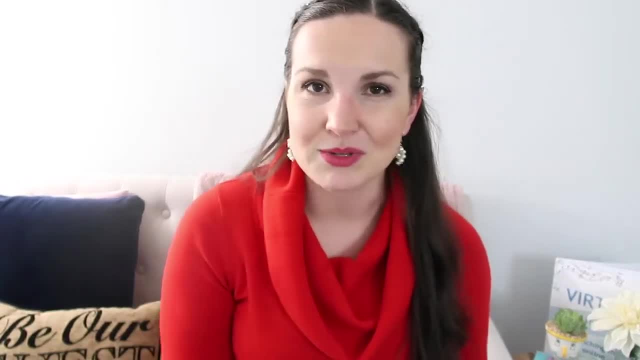 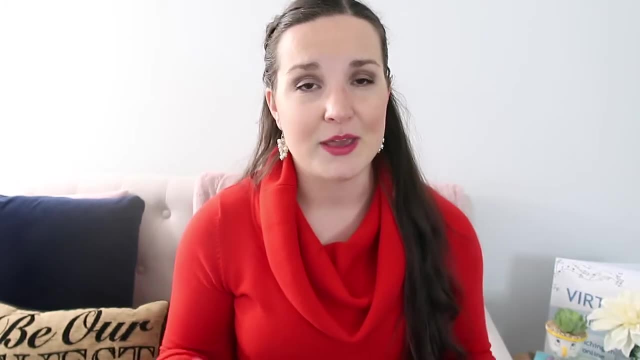 really fun and I just I like that song, They liked the song, so it worked out really well and basically you just assign different drum parts to different parts of your body, So like the drum would be your leg and you would stomp every time the bass drum plays. You can pat your 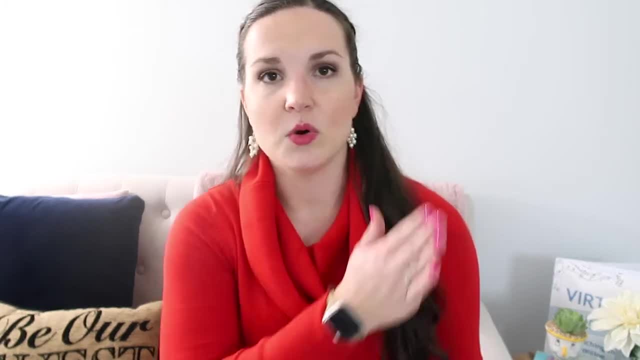 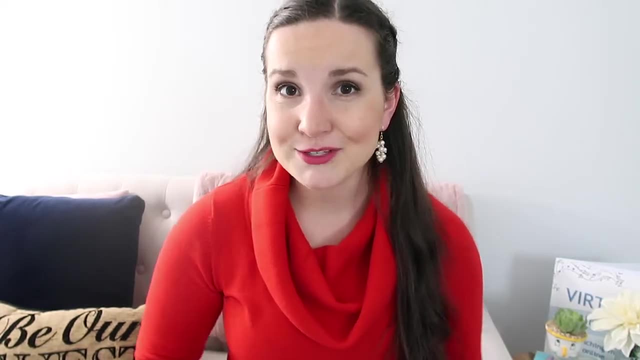 legs for the snare drum. You can do like up here for your hi-hat and different things like that You could click together. if there's like sticks clicking together, All of those things that work just great. and then all you have to do is find like an iconic thing where they have the pictures. 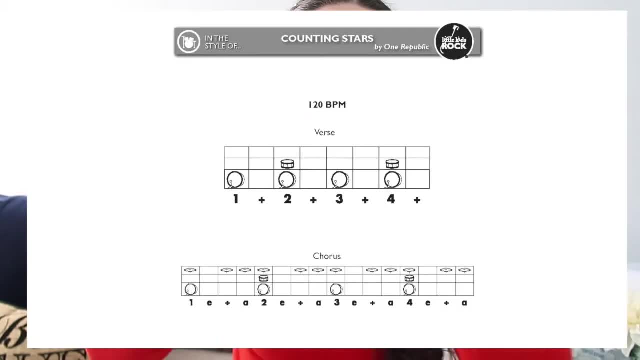 of the drums, so you know what to play. Do you know what I'm talking about? I'll pop one up here and I will also link to it down below, So I get mine off of Little Kids Rock and it just says like: oh the. 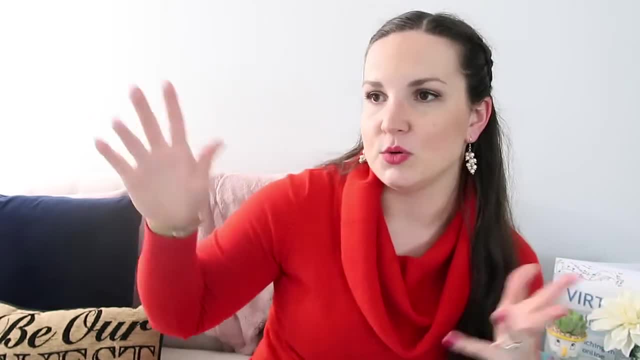 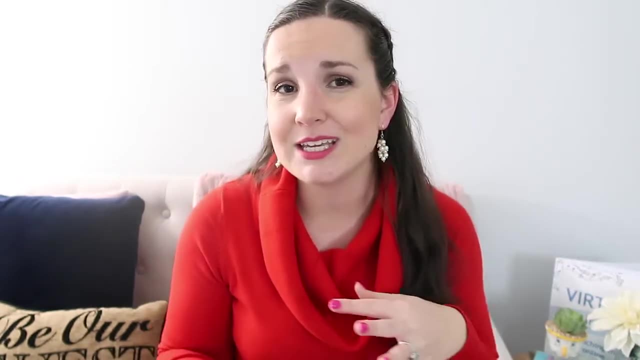 bass drum plays on beat one and the hi-hat plays on beat two and four and stuff like that, and so we just learn it and then we do it along with the song and it's really fun, Really easy way to get them moving without realizing they're moving. They're also playing rhythms without realizing. 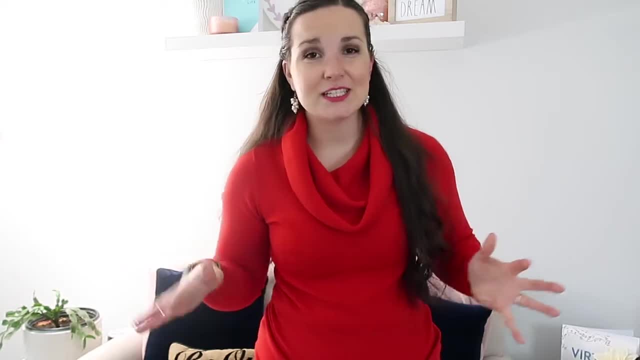 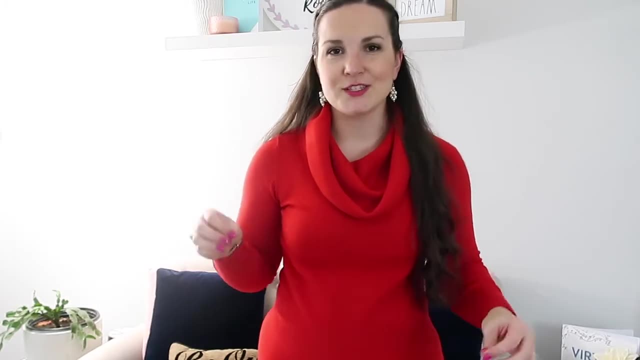 they're playing rhythms and it's just a lot of fun. All right, we had to stand up for the next one, and this is the song: One Bottle of Pop. I learned this actually at a choir camp, and it's just so much fun, and so I love to use this with my fourth and fifth graders, especially in the spring. 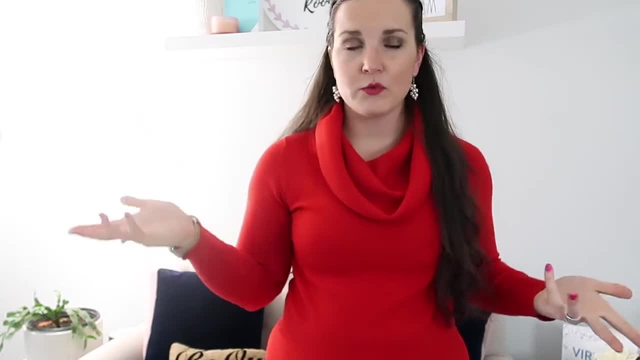 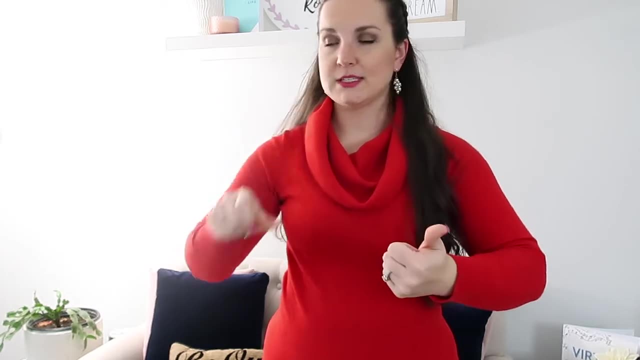 I wanna sing, but I want them to sing, so we do it anyway. so I will sing the whole thing before you and show you the actions. The first one is I always say thumbs up, thumbs to the side, and that's how we start. and it goes like this: 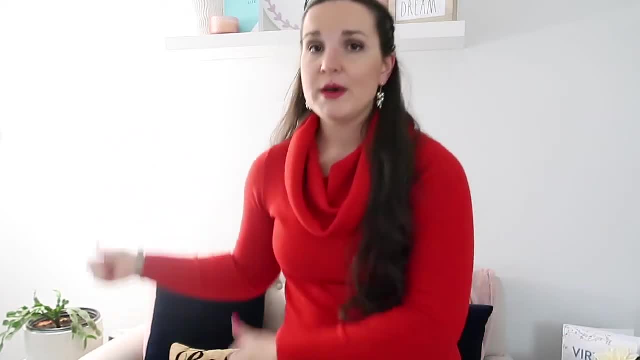 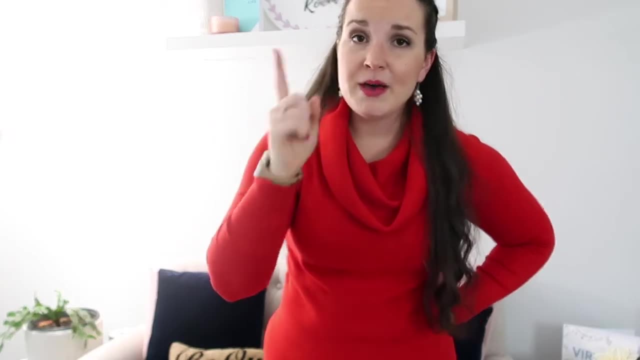 One bottle a pop. two bottle a pop. three bottle a pop. four bottle a pop. five bottle a pop. six bottle a pop. seven bottle a pop pop. don't throw your trash in my backyard, my backyard, my backyard. don't throw your trash in my backyard, my backyard's full. 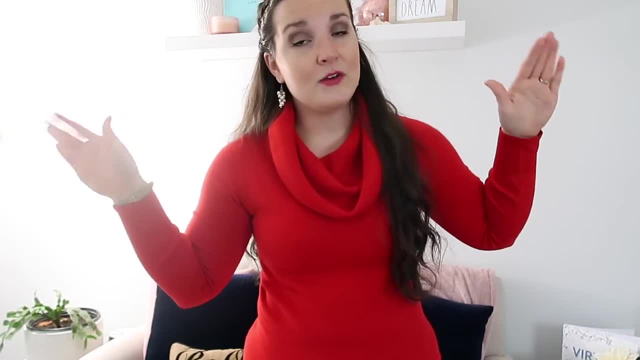 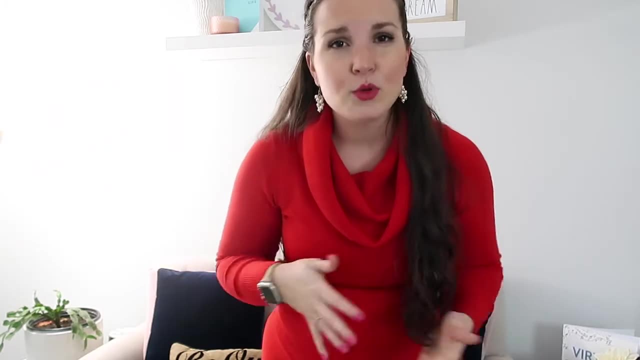 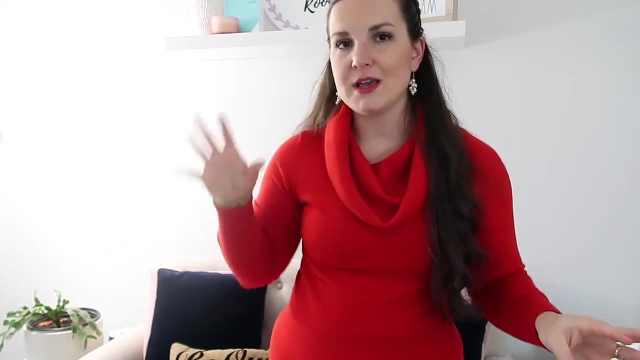 Fish and chips and vinegar, vinegar, vinegar, fish and chips and vinegar, vinegar and pop. so really really easy, really simple movements, really simple song, but it's a lot of fun. then we like to take it up a notch and make it into a round, and i like this for a round because the different sections are so different that it's 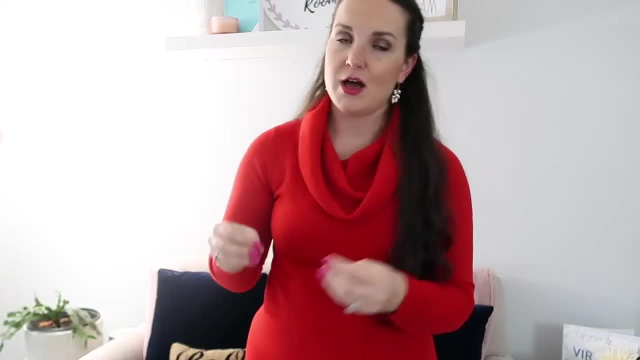 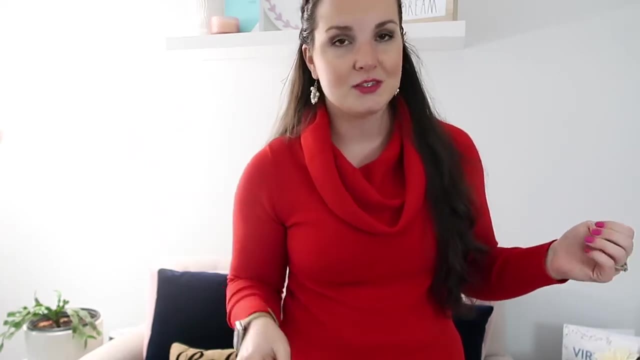 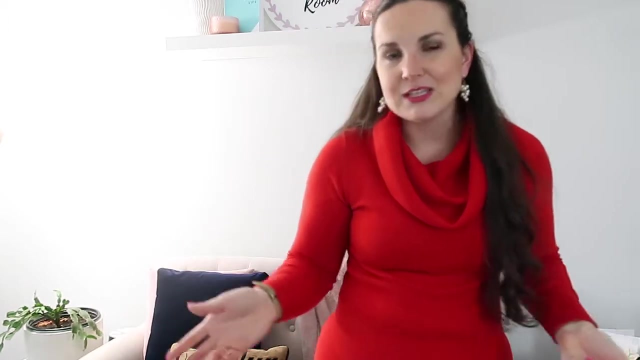 easier for them to stick to what they are supposed to be doing on their section. we've also done a song on zoom teaching online. i just, you know, hit the mute button, so it's sad you can't hear them, but they do really like it because it's just kind of fun and it's easy- little movement activity. so 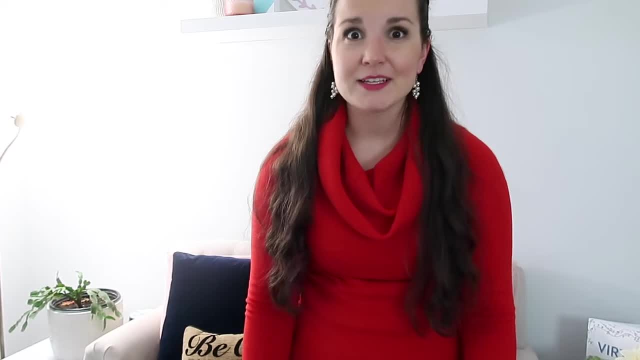 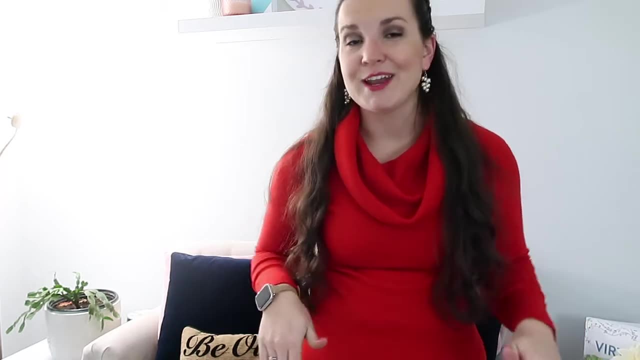 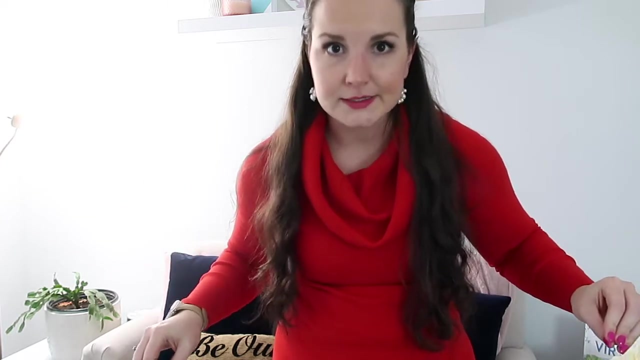 there you go. another one we have to stand up to talk about and that is pizza, pizza daddy. this song i found by chance and it is a hit. it is so much fun. so what you do is you sing this song and then the magic part is when it says pizza, pizza daddy. yo, yes, i said that. right, you are. 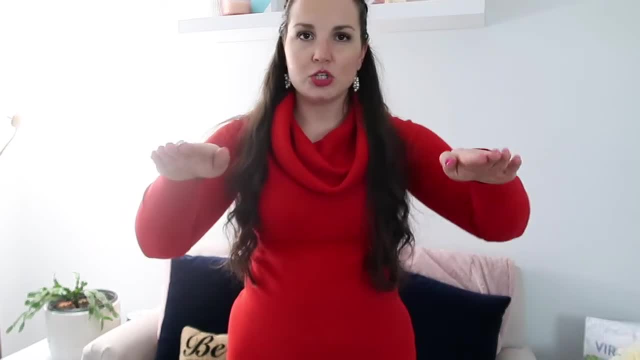 moving your feet in and out, which the kids just think is hilarious. so i'll show you with: oh, you can't even like, you can't even like, you can't even like. see my feet. so what is the point of standing up? i don't know. um, so what the hell? i'll back the. 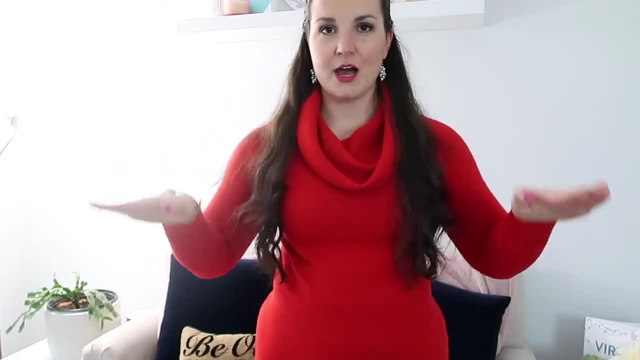 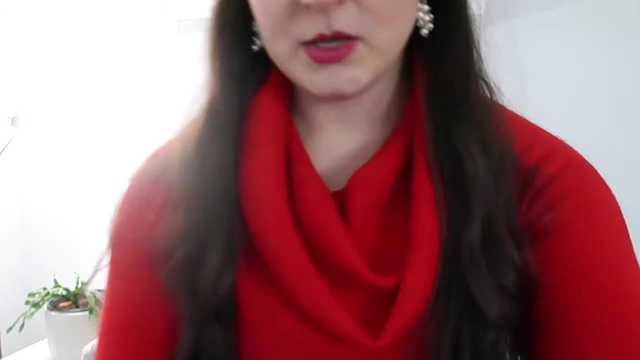 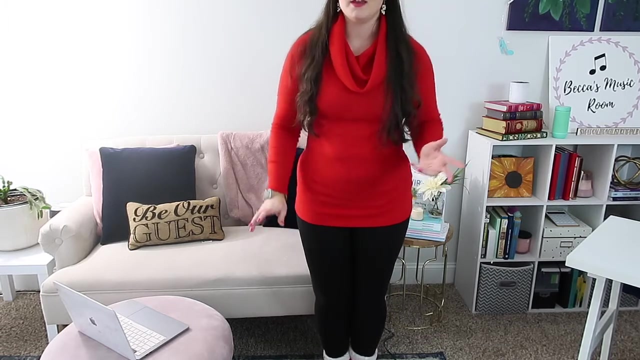 camera up in a second, but basically it goes um. i always say: out cross, out, cross together is the pattern. let me back you up so you can see. all right. so our pattern is: out cross, out, cross together. and then we go again and out cross, out, cross together. so that happens every time you. 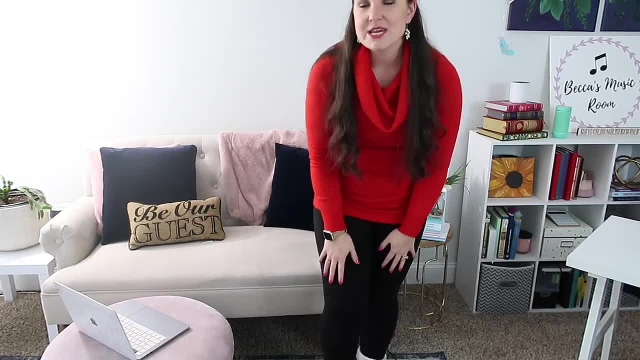 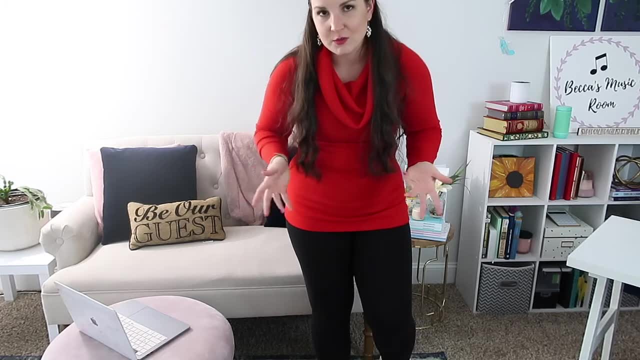 say pizza, pizza, daddy yo. so i'll sing the song. um, the beginning is supposed to be: annie has a boyfriend. i always just do, friend, because i feel like that's a little bit. you know better. i really don't want to encourage them to have boyfriends when they are. 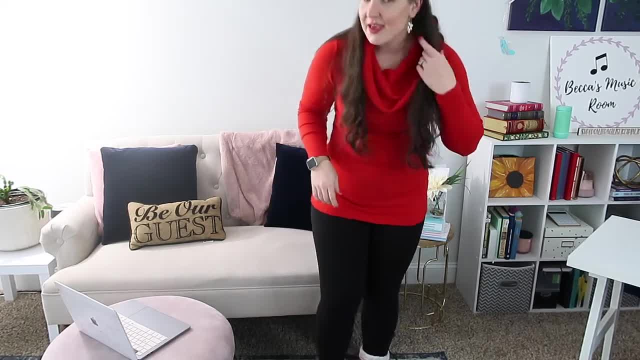 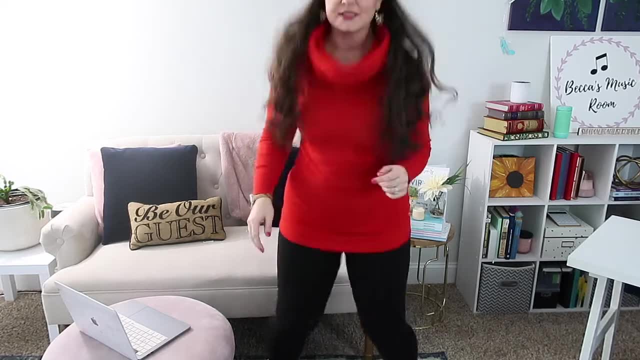 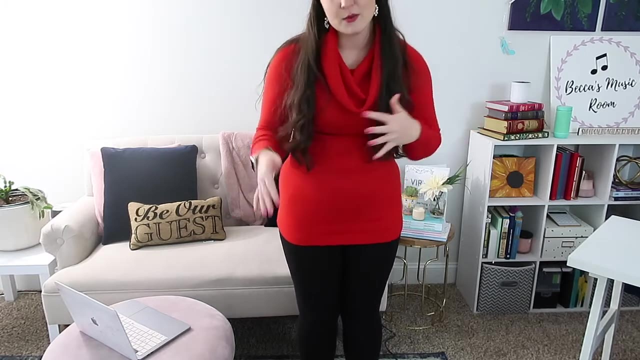 in fifth grade. so here we go. um, annie has a friend: pizza pizza daddy yo. how do i know it? pizza pizza daddy yo, because she told me: pizza pizza, daddy yo. now how you play this is one person comes up to the front or in the middle of the circle. 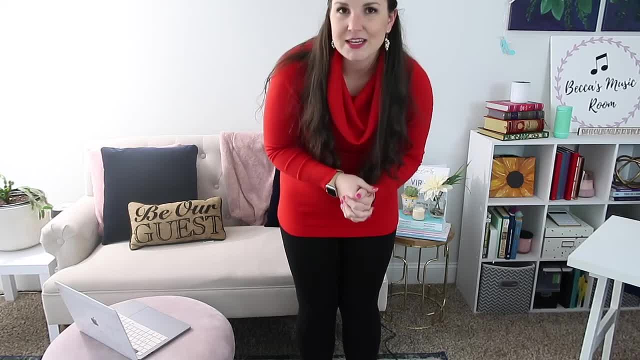 and then you have to say: out, cross, out, cross, out, cross together. and then you have to say out cross, out, cross together, and you put your their name in instead of annie. and then can you even see my head? you put their name in instead of annie, and then after that you get to have them pick what you're gonna do. 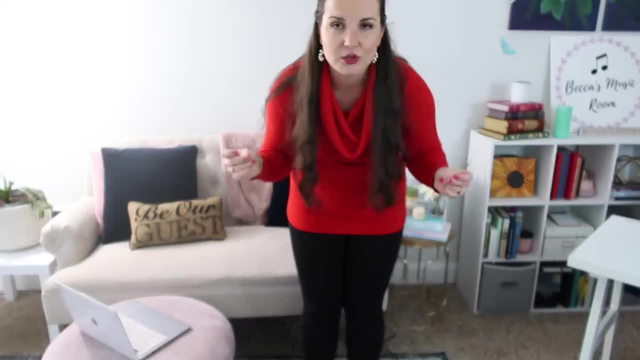 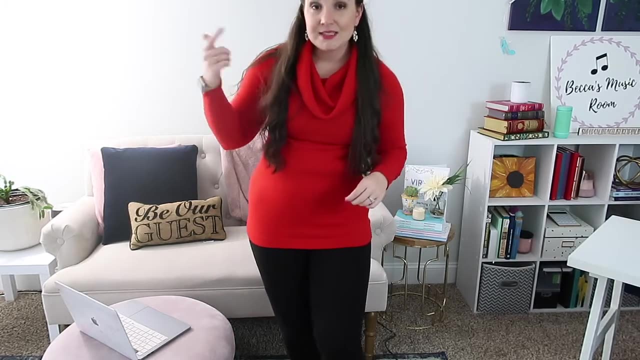 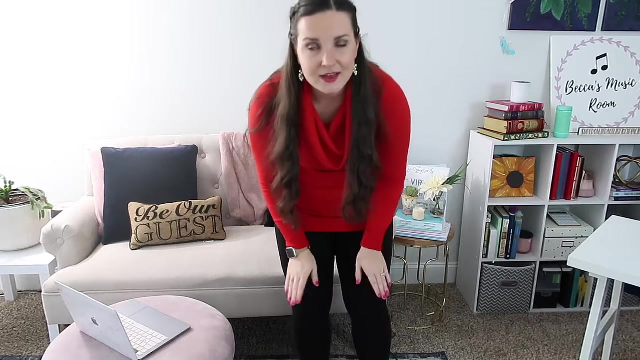 so, um, i usually have them do two actions. so they'll do like snap it, and then like pet. we'll do those two. so the person up front calls out what they're gonna say. so they'll say: let's snap it. and then we all go snap it. snap it, daddy yo. and they'll say: let's party party, daddy yo. and then they'll say: 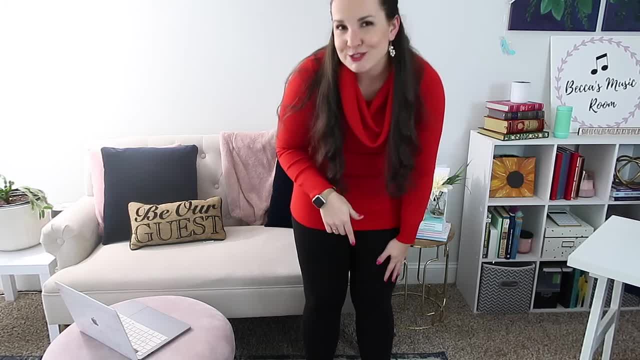 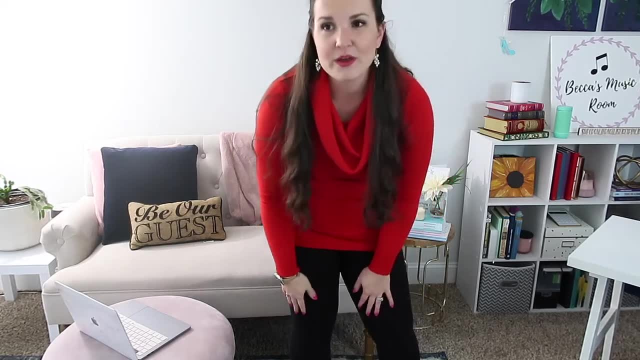 let's end it and they're supposed to cover their eyes and turn around in the circle and then whoever they are pointing to is the next person to go. but honestly, i usually just have the kids raise their hand if they want to go and then they pick someone with their hand up who hasn't gone before, because 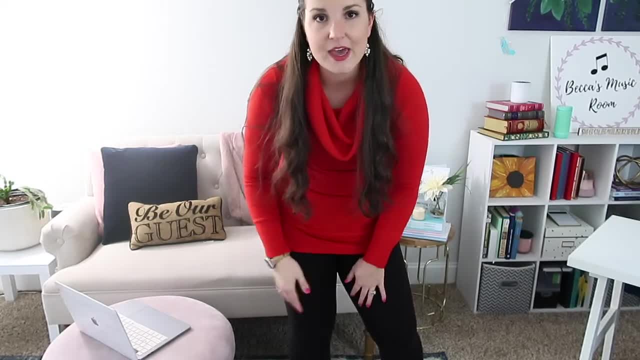 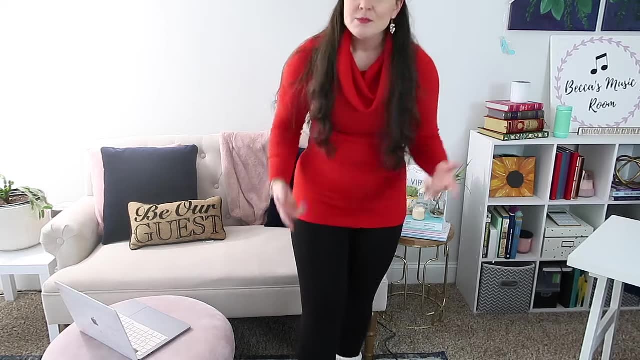 it's easier. so i'm gonna run through the whole thing and i'll say: miss davis, because i'm the one doing it and i always do it a couple of times myself to show them lots of different things that they could do. so it goes like this: miss davis has a friend, pizza, pizza, daddy yo. and then i'll say: 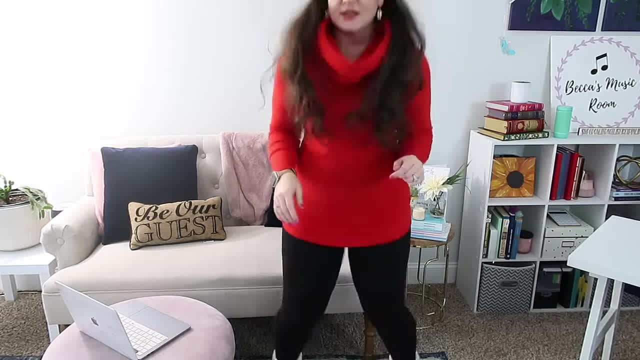 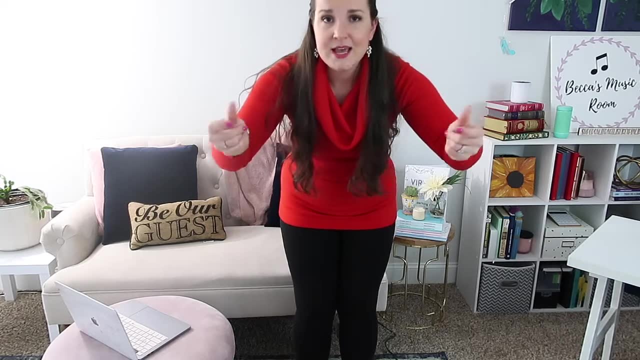 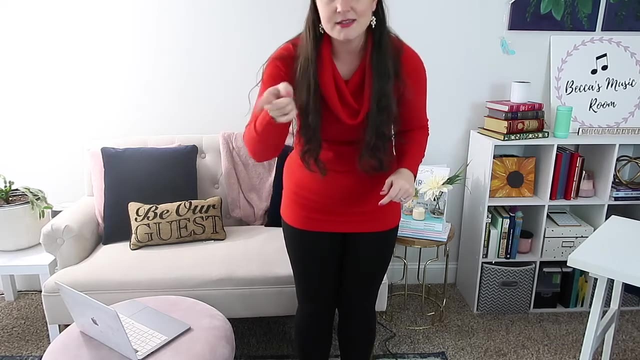 pizza pizza, daddy yo. how do i know it? pizza pizza, daddy yo, because she told me: pizza pizza, daddy yo. let's snap it, snap it, snap it, daddy yo. let's stomp it, stomp it, stomp it, daddy yo. let's end it, end it, end it, daddy yo. and then you repeat again with the next person. i know it sounds so, so. 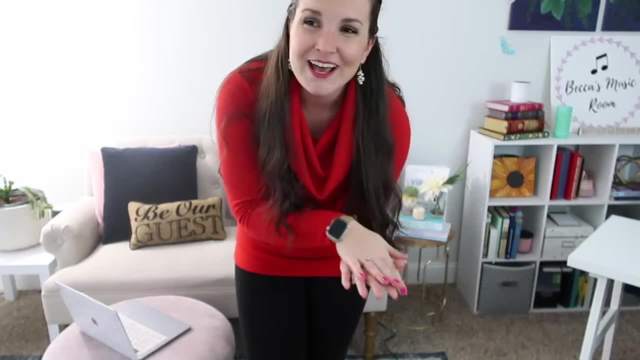 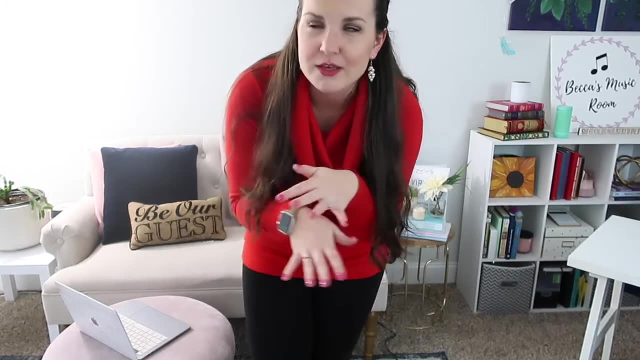 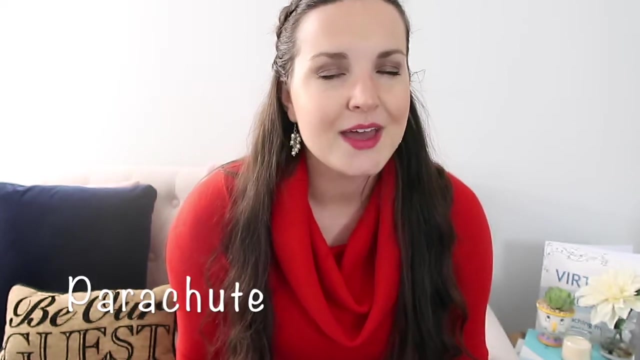 silly, but it is so much fun and even the like, toughest, coolest you know boy fifth graders are like i'm too cool for this. have so much fun, all right. the next thing is anything that goes along with a parachute. if you don't have a parachute in your classroom, i 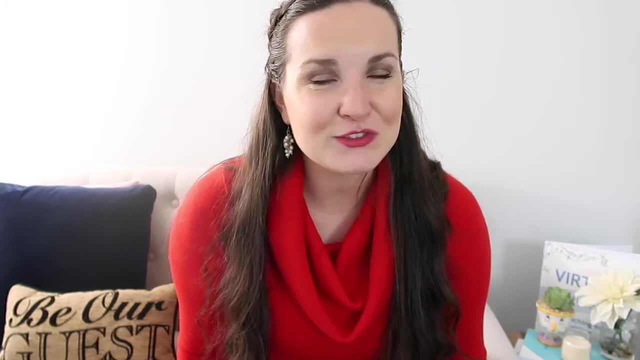 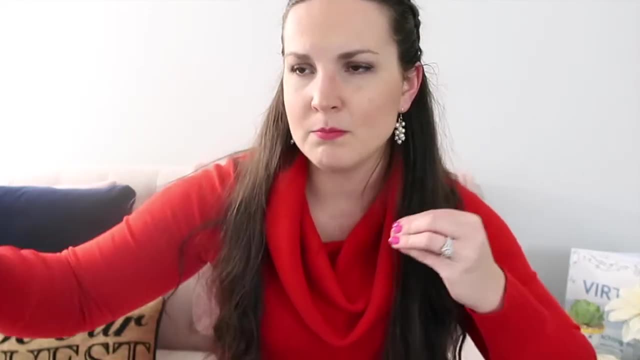 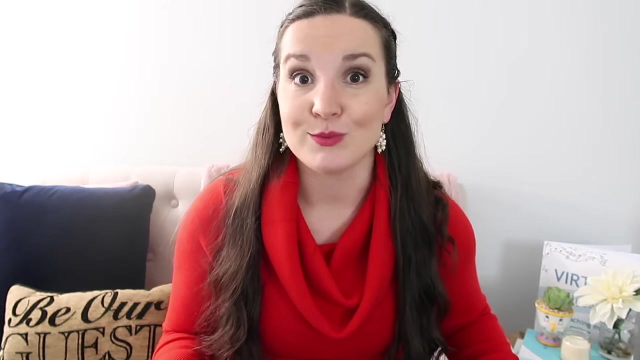 highly recommend that you get one. they are so, so, so, so much fun. so we do this with- oh, i don't even know the- i think it's just the star wars theme- the bomb, that one, and so at the beginning we do like little tiny shakes and then, once it actually starts with that part, i just sang for you. 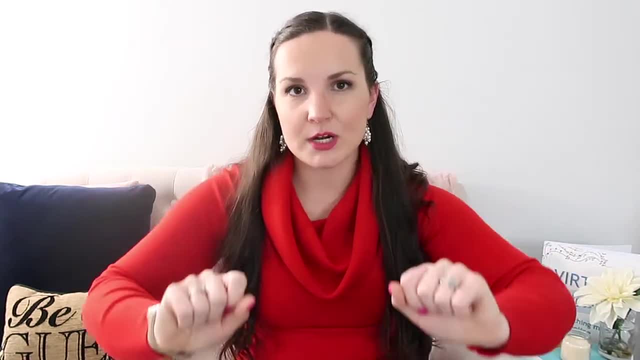 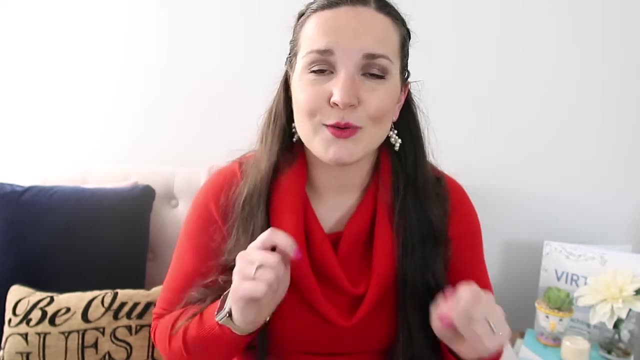 then we go up for four nice and slowly and then down for four nice and slowly on the b section. i have them walk in a circle to the b section and then at the end we just go back to those little little shakes. so easy, easy, easy peasy, you can do it in like one class period and 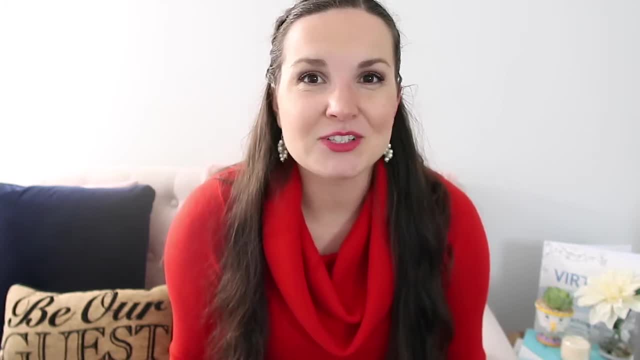 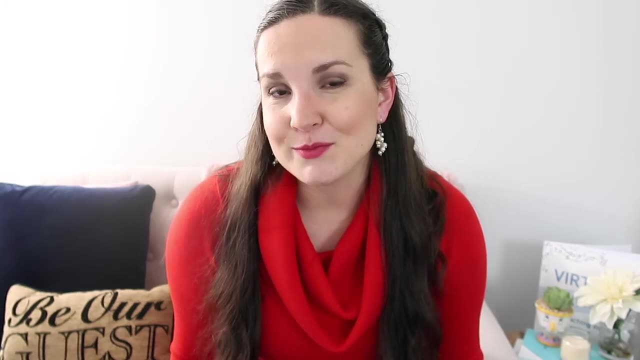 it's so much fun. so much fun, i promise. and also the kids who like star wars will be like: this is star wars. i'm like, yeah, it is. it's so great, isn't it now, obviously, if you're watching this when this comes out, it's not an option, because you're probably either virtual or you're not. 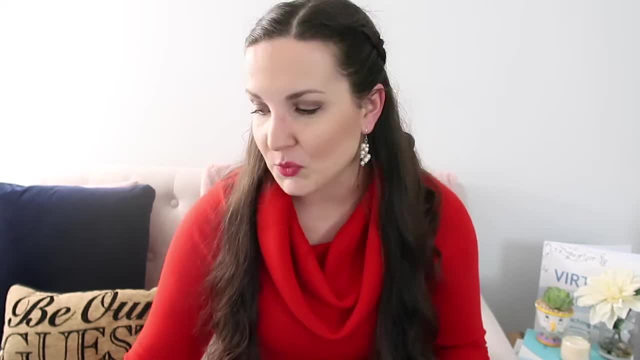 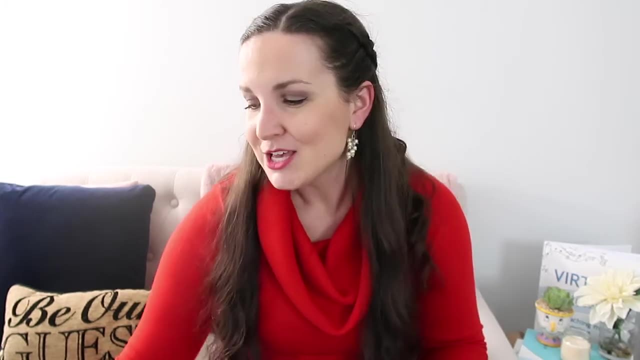 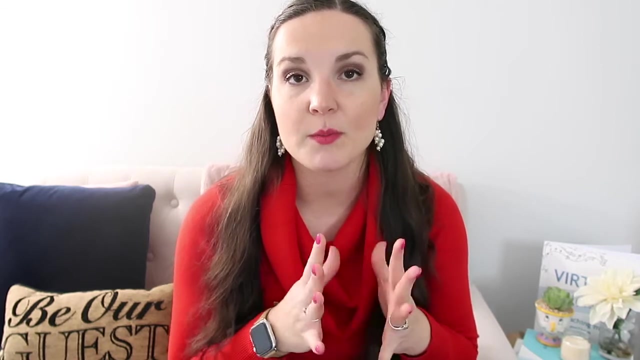 watching other things or having kids closer than six feet away. but eventually i believe that it'll go away and you'll be able to use the parachute again, so i did not make up that um routine. i will link it down below and i will also link the arty almeida book parachutes and ribbons and scarves. 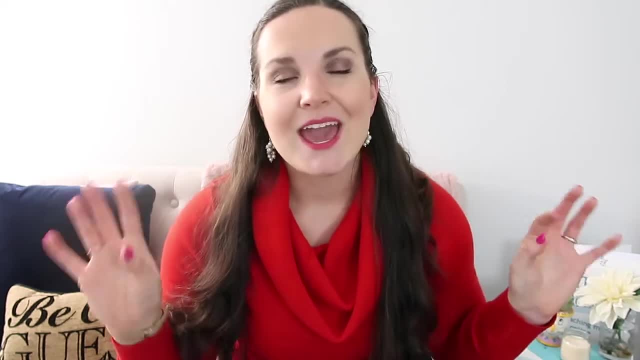 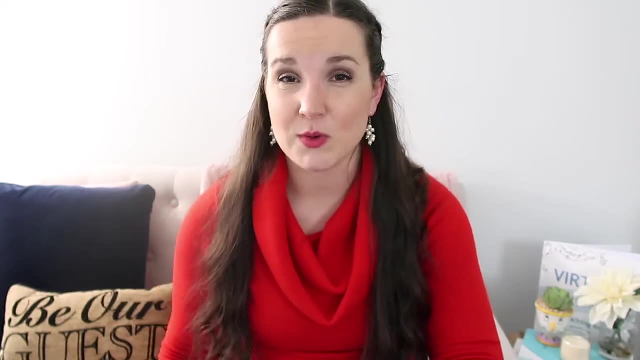 or scarves and parachutes, i don't know- those three things in some kind of order. and it is my absolute favorite book. it is so much fun. i use it with all of my classes and it's just. it's great. i use it all year round, so definitely check that one out as well. all right, the next one is the. 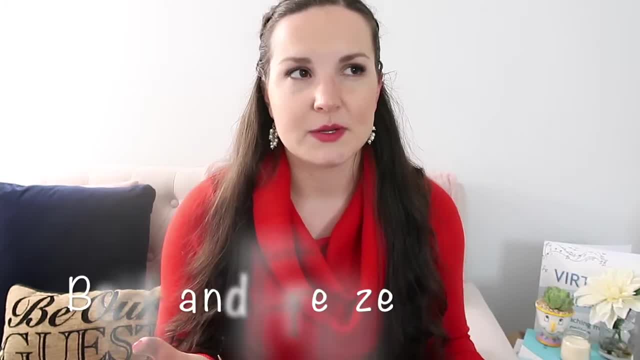 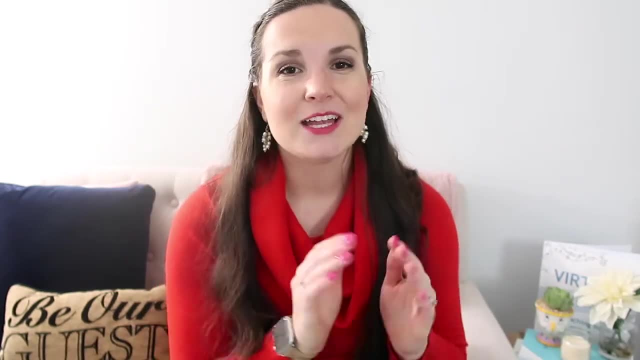 next one is super, super easy and i call that beat and freeze, or sometimes i call it statues, i don't know, i call it different things. basically, i take a drum and i play eight beats on the eight. eight beats on the drum, and the first one is louder than the rest. what they do is on the 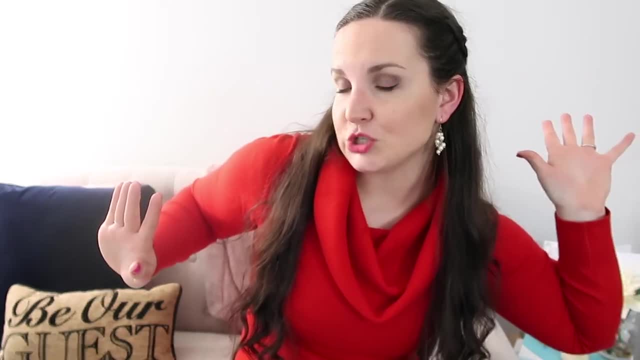 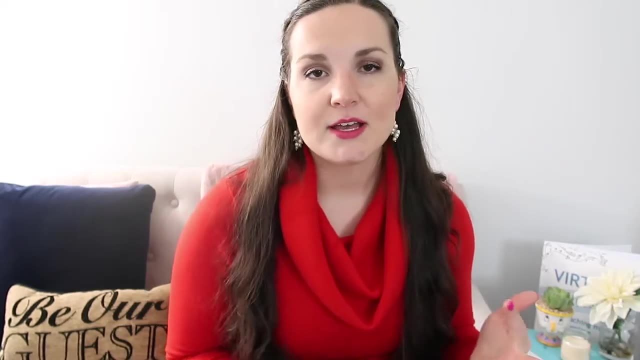 loud one. they have to make a post like a statue and then they hold it and then the next time we get back to your downbeat, then they pick a different pose. so this allows them plenty of time to think about it as they're going. i like to change the tempo, so we'll speed it up. we'll. 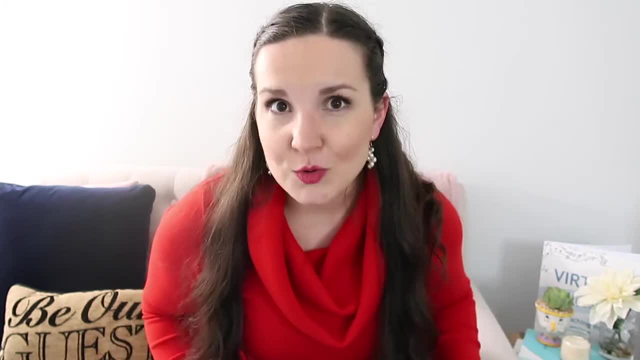 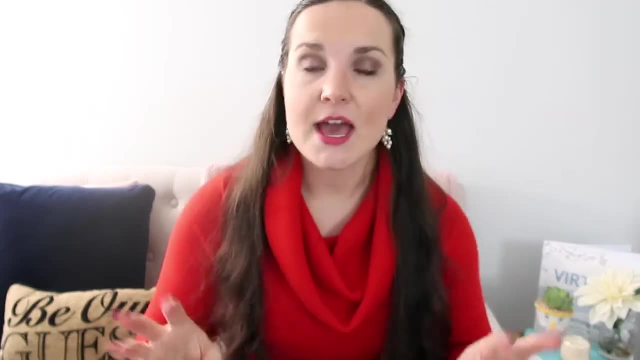 do just all these different things and it is so, so much fun, especially when we start getting faster and then i just start playing all of them loud and so they're like it's hilarious and also so much fun. if you have kids who are a little more shy about moving and stuff, i tell them 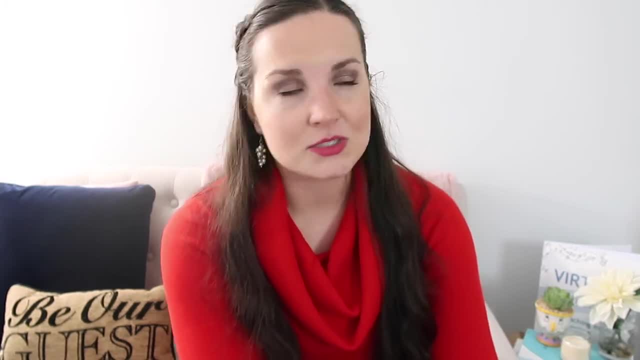 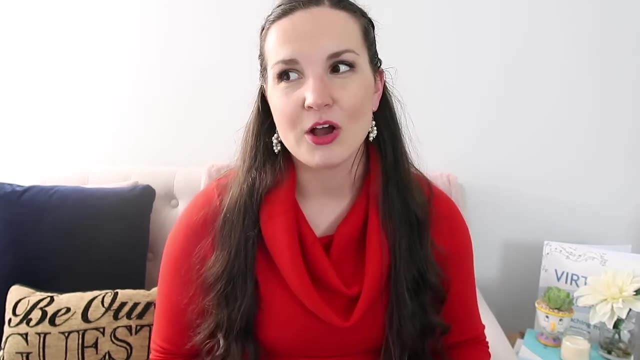 you don't have to do anything fancy, but you do have to move. so even if it's just like, like that counts, you just gotta do something. and so i have them all. they all get like, they get really into it, like, really into it. it's hilarious and 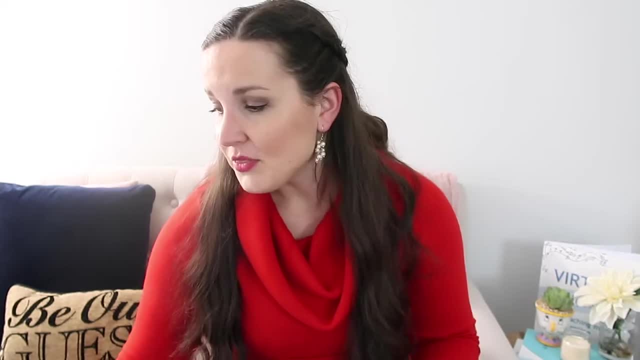 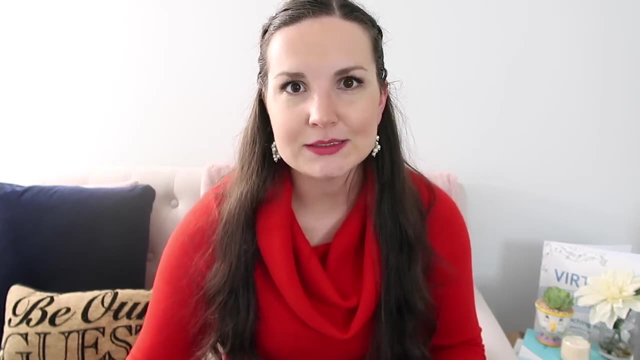 so much fun and you can totally use that with any grade. the next one is: i guess it's not really a movement song, but i wanted to include it because it's so much fun. so this is a singing game that, again, you can't play now but you hopefully will get to play in the future. if you're watching this, 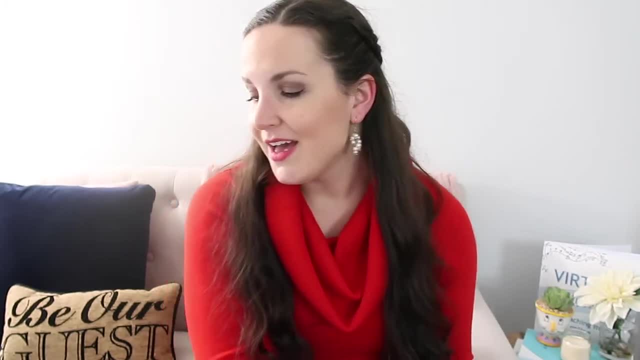 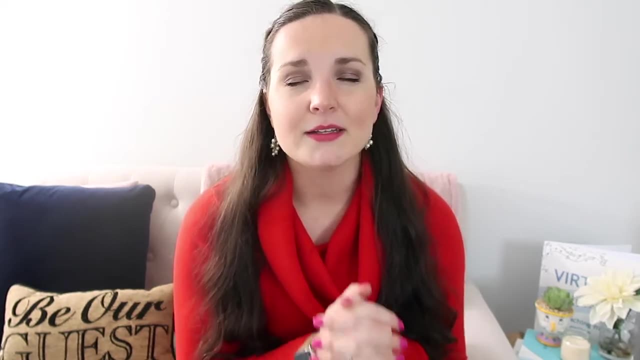 future. you're like, oh, i remember those days and i'm glad they're not here. um, so this is a quack quack. this is an israeli beat passing game that i use with my fourth and fifth graders, and they love it. it is so much fun, so the song goes. 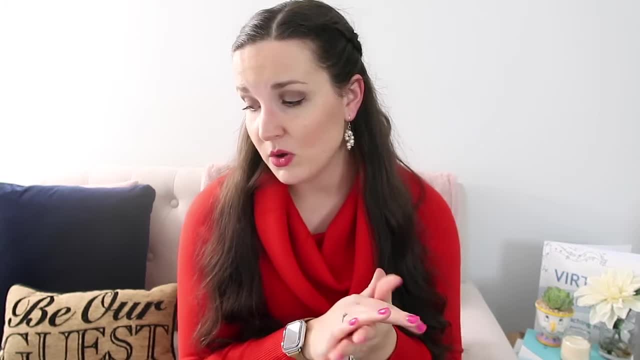 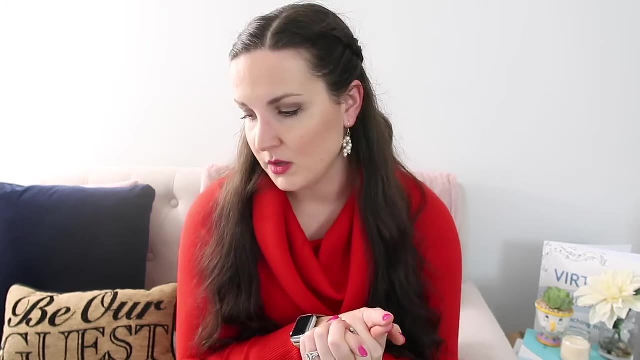 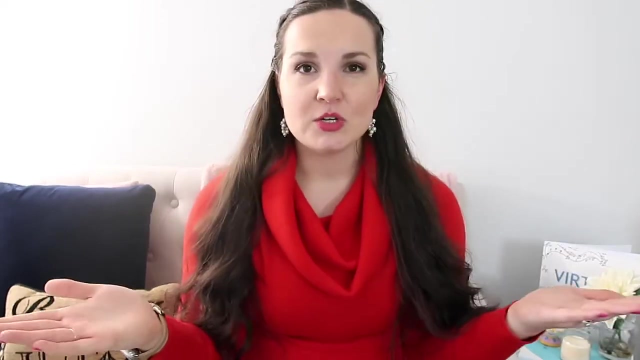 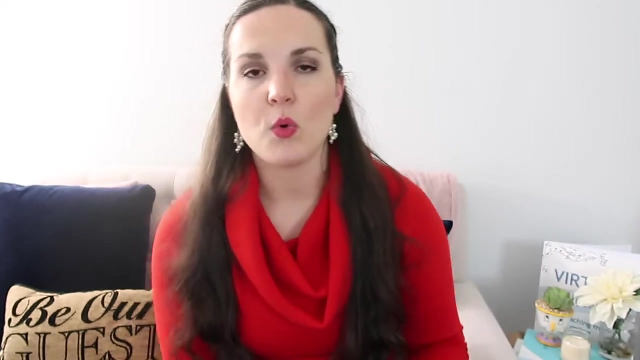 one, two, three, four, five, sorry, um anyway. so all they do is they say: and they have one hand on top of the person's over here, one hand underneath the other person's here, and they pass the beat in a circle while we sing, and then whoever gets landed on on on five is the person that's going to sing the song. 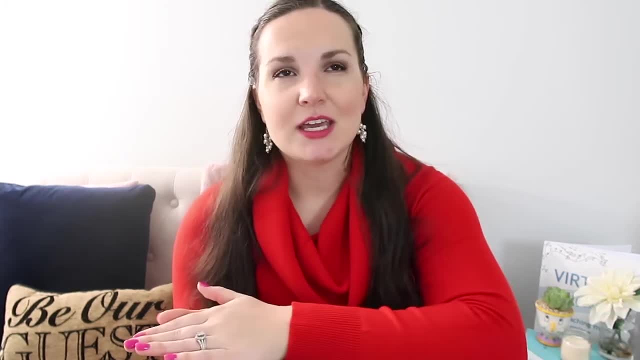 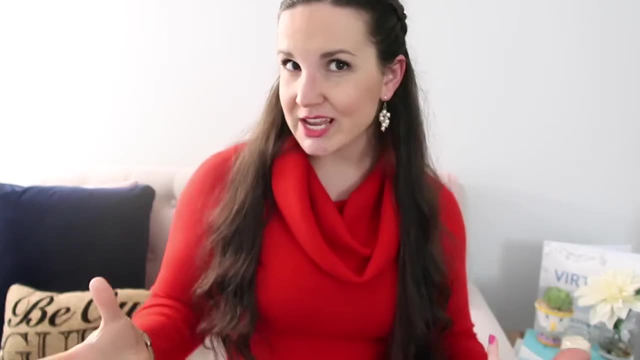 and then the person who's out. it's not really moving because you're just like moving your hands, but it is a lot of fun and it injects kind of the same energy that movement does, because there's just like a energy that you get in the room when all the kids are dancing and stuff like that. that. 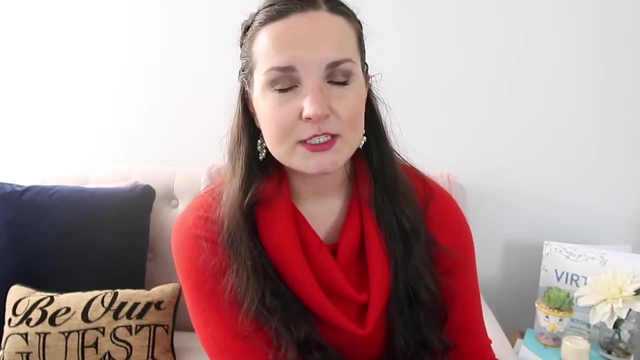 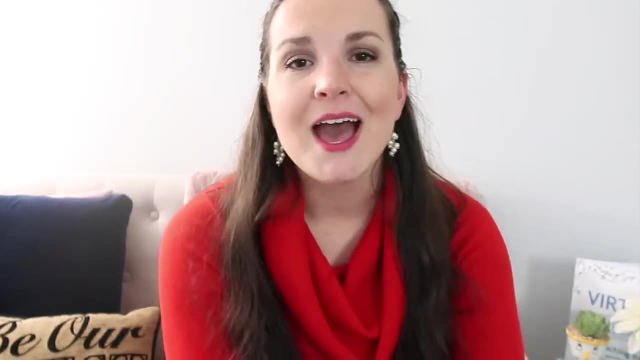 you get also when you're doing this. all right, so that's all for my list for today. i do have a lot more that we could talk about, but i'm gonna end it here. you might be like becca: you didn't mention folk dancing. i know i did that on purpose. i purposely didn't know that you were gonna do that. 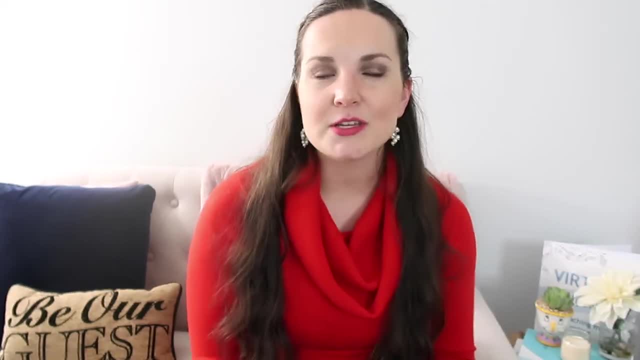 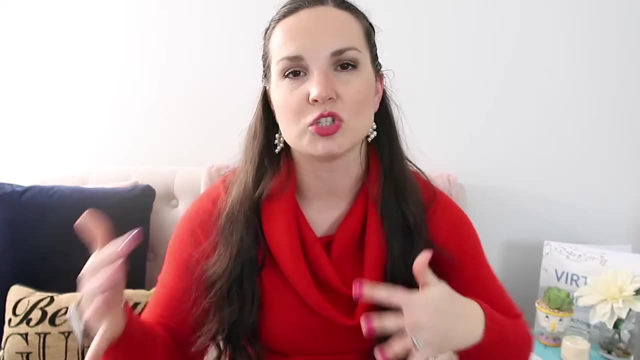 did not mention any folk dances because i feel like that's an easier thing to find than just like: oh, i want a quick movement activity versus like oh, we're gonna learn a folk dance. like. those are just very different things, so maybe we'll do a different video with my favorite folk dances. 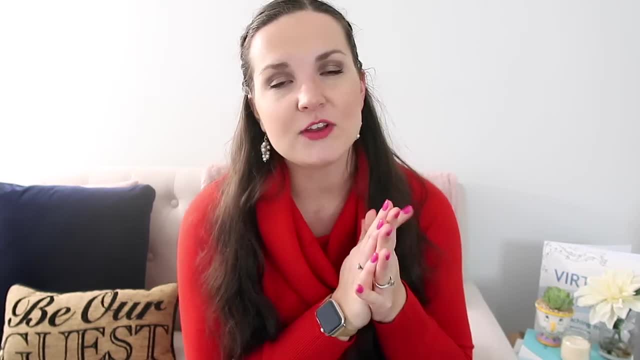 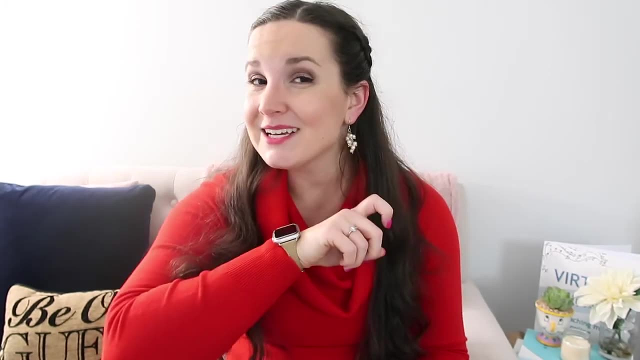 let me know if you'd be interested in that. if you made it all the way to the end of the video, i would love to know your favorite movement activities for fourth and fifth grade down below. thank you so much for watching. hit the like and subscribe and i will see you next time. and yes, 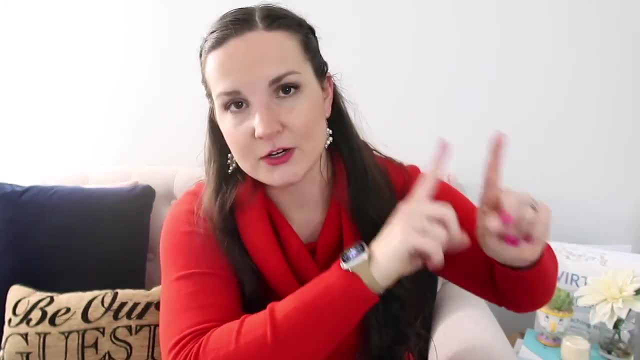 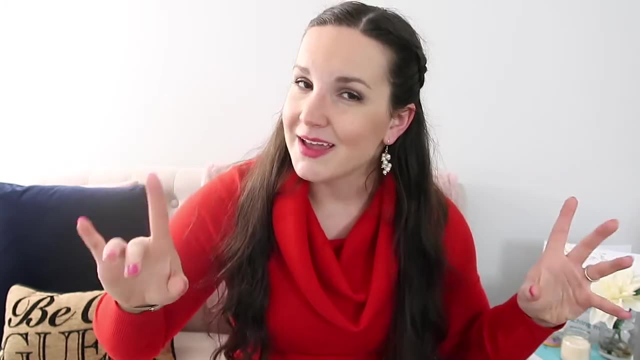 there will also be second and third grade and first and second nope kindergarten, first grade and second and third grade versions of this video. so again, hit the subscribe button so you don't miss out. thanks so much for watching and i'll see you next time. bye. you.